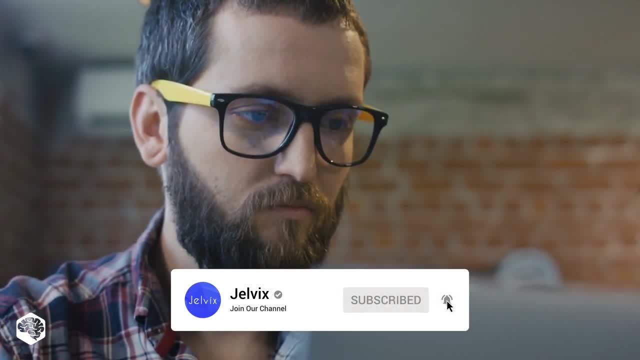 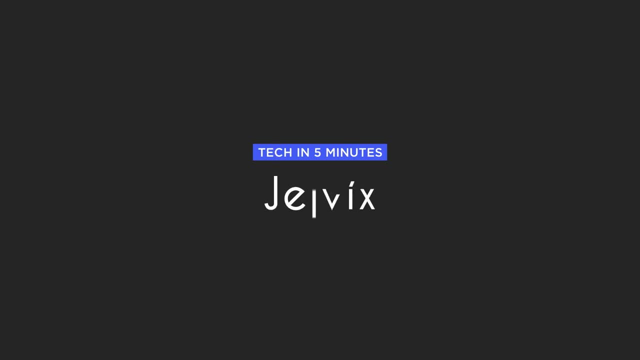 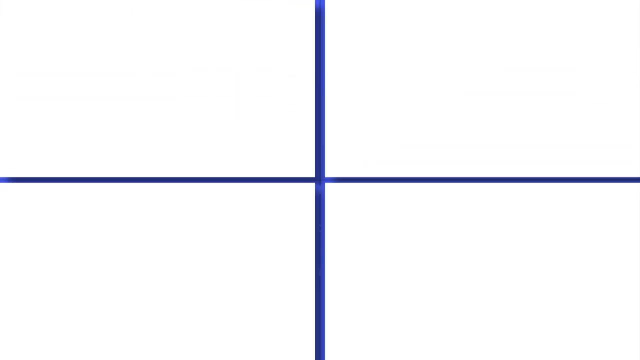 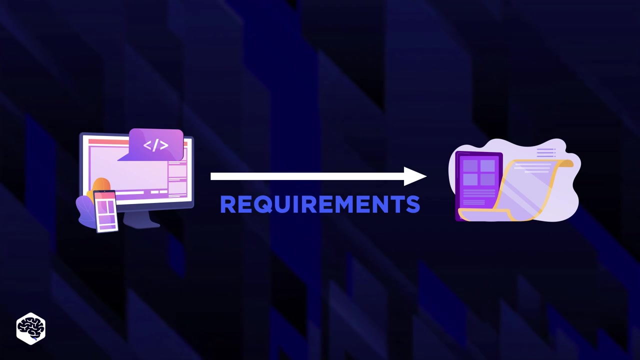 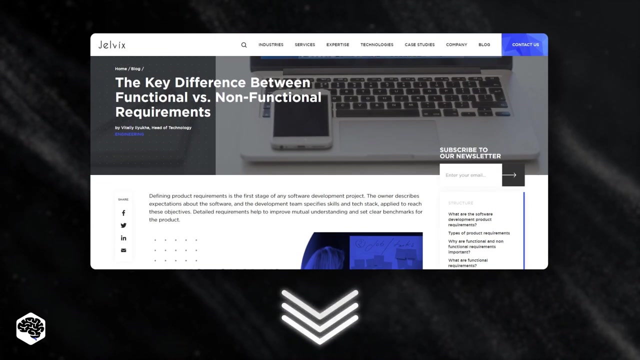 thoughts on recent developments in the tech industry. Subscribe to never miss new videos. Let's start. We need to measure quality to check if the software solution satisfies its requirements. The requirements can be classified as functional or non-functional. Read our comparison of functional versus non-functional requirements for more details. The link is in the description box. 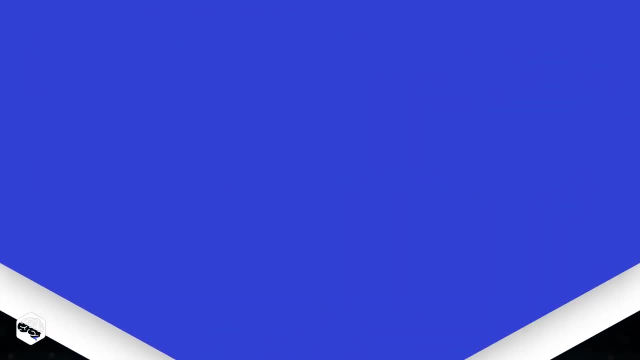 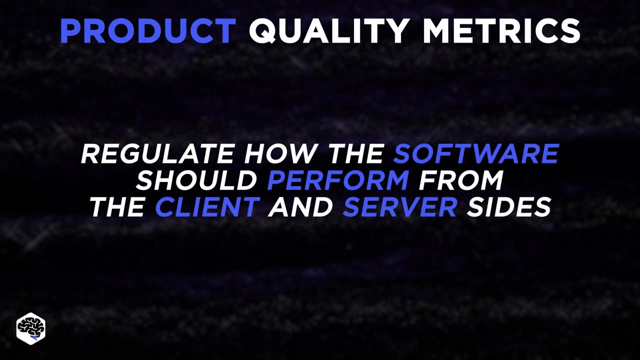 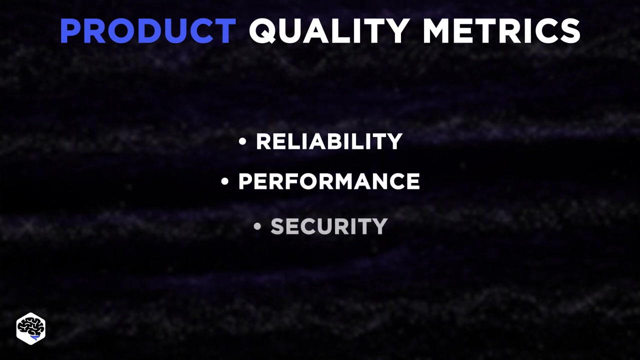 Let's now review the major types of software quality metrics. The first group is product quality metrics. They regulate how the software should perform Both from the client and server sides, And this group includes such components as reliability, performance, security and maintainability. The second group is code quality metrics. 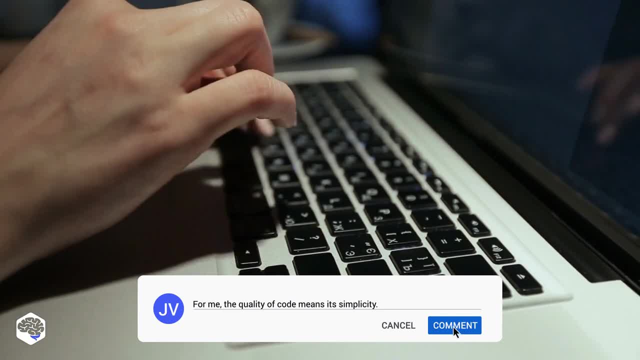 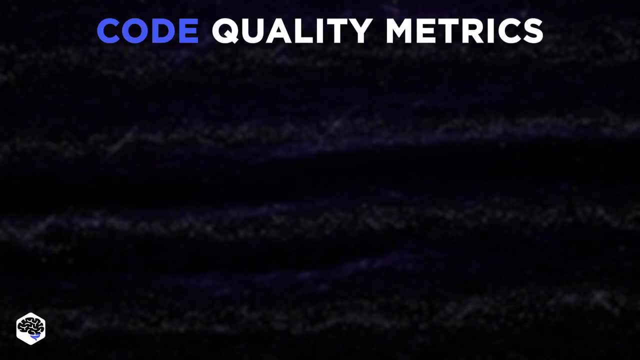 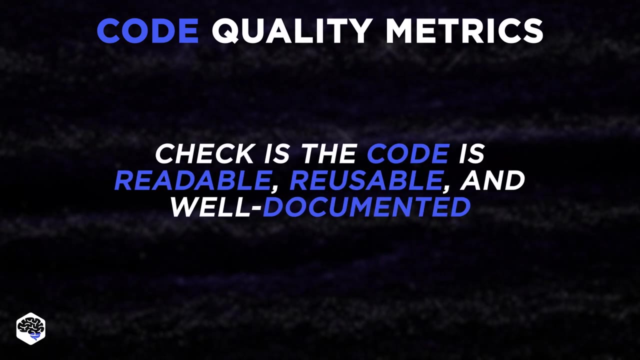 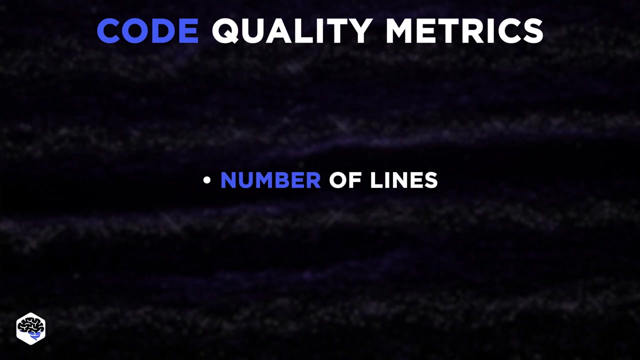 How would you check the quality of code? Share your thoughts in the comments section. In fact, it is difficult to create code quality metrics. Still, we at Jelvix think that good code, written according to the coding standards, is readable, reusable and well-documented. So the criteria for measuring code quality include number of lines. 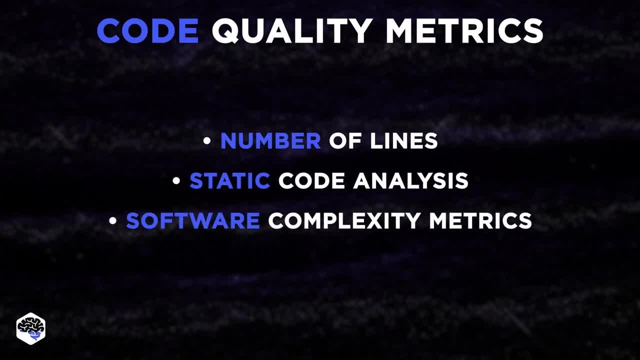 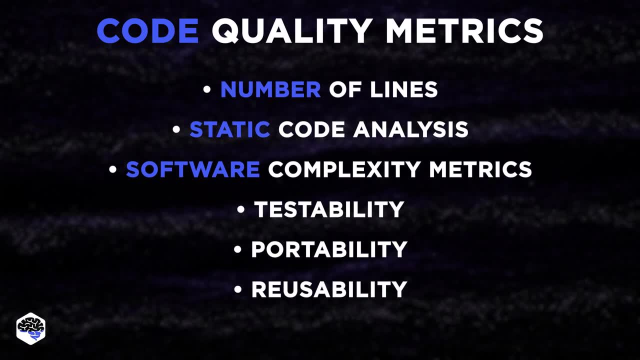 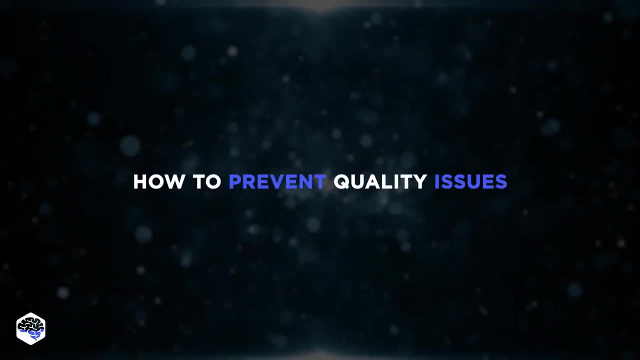 static code analysis software complexity metrics, as complex code is more difficult to maintain testability, portability and reusability. Now we are coming to the important question: How to measure software quality and maintain it. It is always easier to prevent the issues by 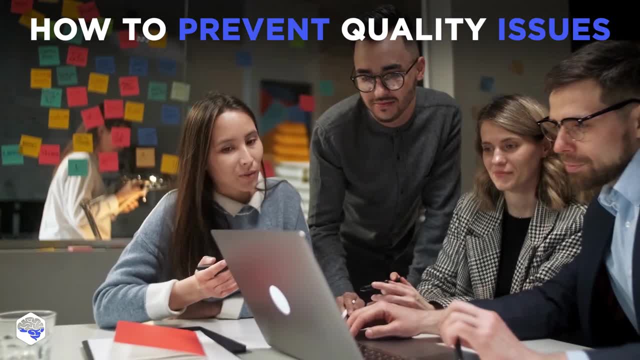 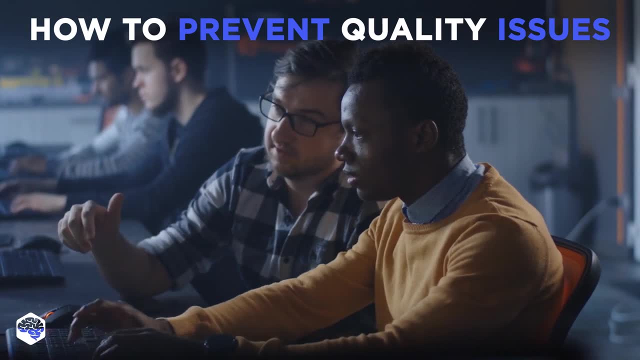 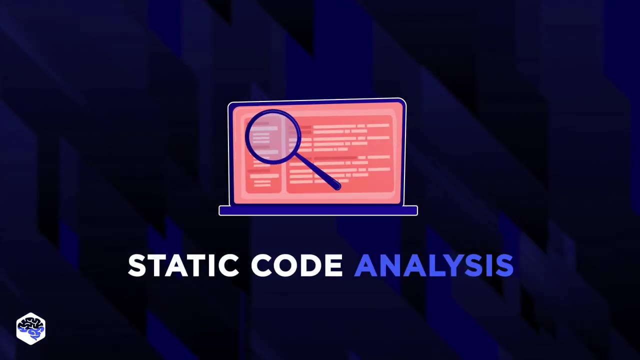 releasing high-quality software than to deal with the errors that come out after the release. So keep watching to know about the practices the Jelvix team uses for delivering high-quality software solutions. Among development, best practices are: static code analysis: It examines the code without launching it and checks it according to the coding standards. 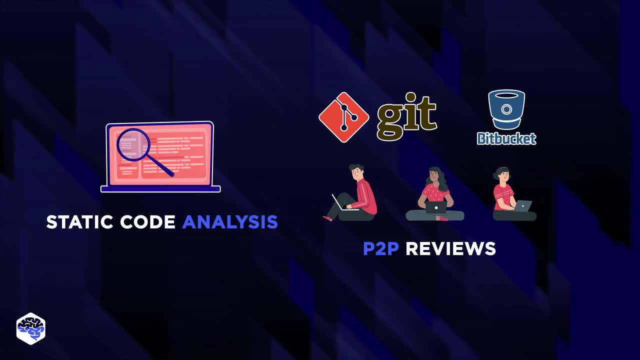 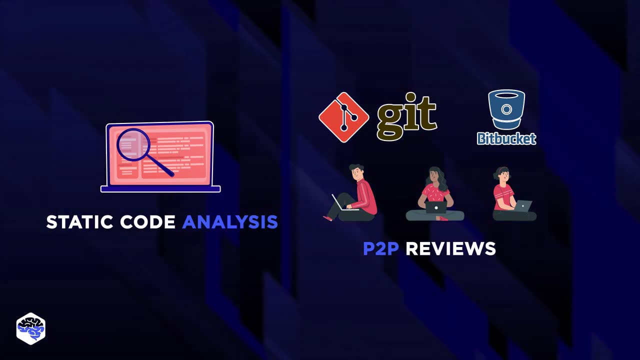 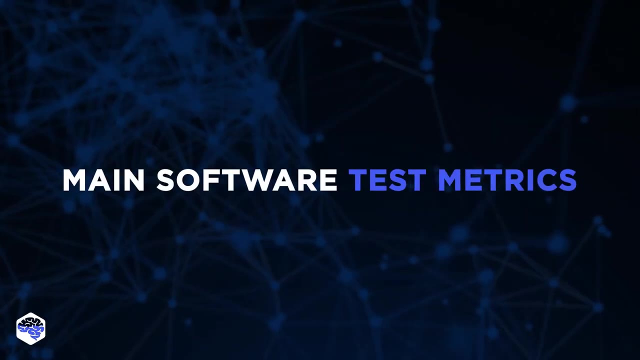 P2P reviews. We use Git and Bitbucket for version control and remote repository management. When the feature is completed, the teammates act as code reviewers. Finally, we conduct reviews by senior or lead developers. So what are the main software test metrics we use?